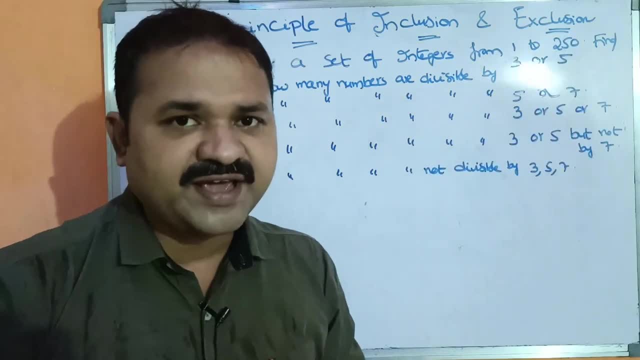 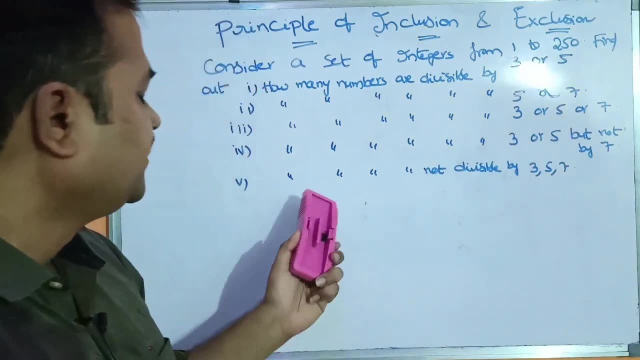 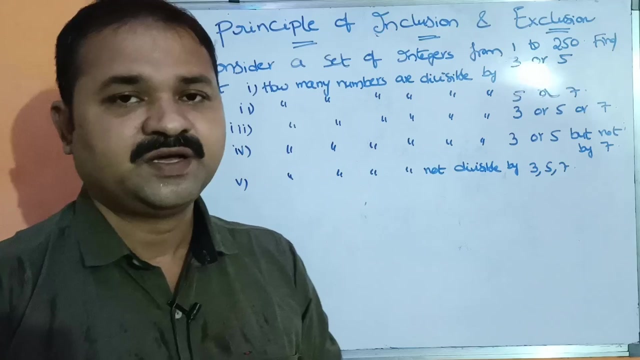 how many numbers are divisible by 3 or 5?. Next, how many numbers are divisible by 3 or 5, but not by 7?? And the last problem is: how many numbers are not divisible by 3 or 5 or 7?? So let us solve all these examples. So first here: 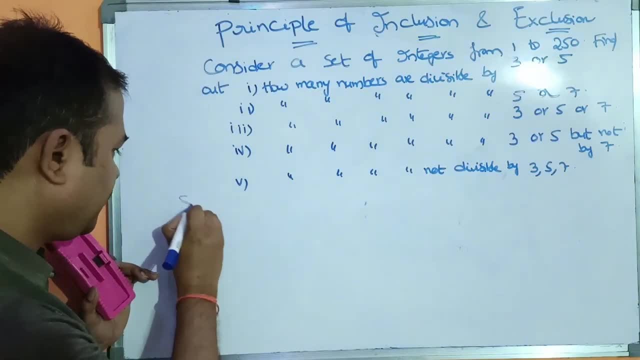 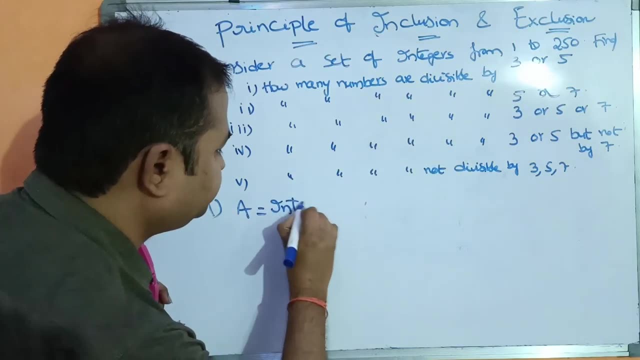 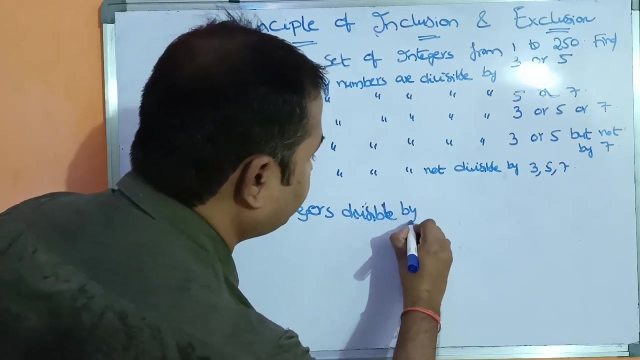 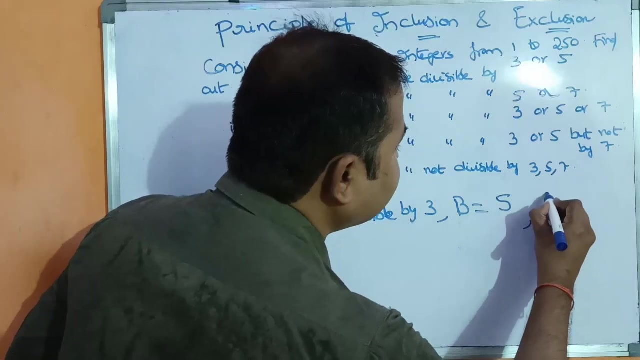 three numbers are given: 3,, 5, 7.. Solution let: a is equal to integers divisible by 3.. Integers divisible by 3, divisible by 3.. And b is equal to integers divisible by 5.. C is equal to integers. 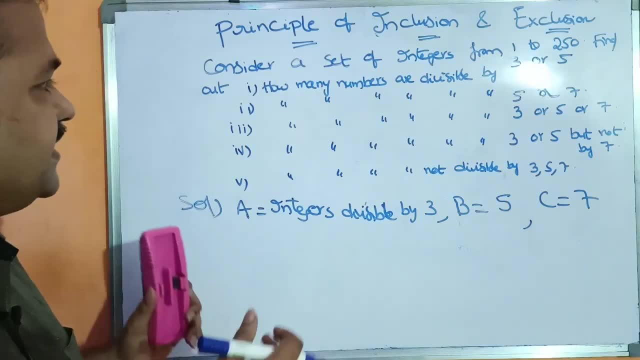 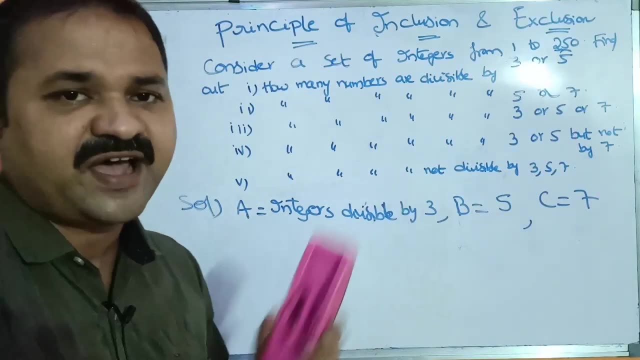 divisible by 7, okay, Next. so here, what is the maximum number? 250 is the maximum number. So first let us find out n of a, n of a So, n of a means, n of a means. 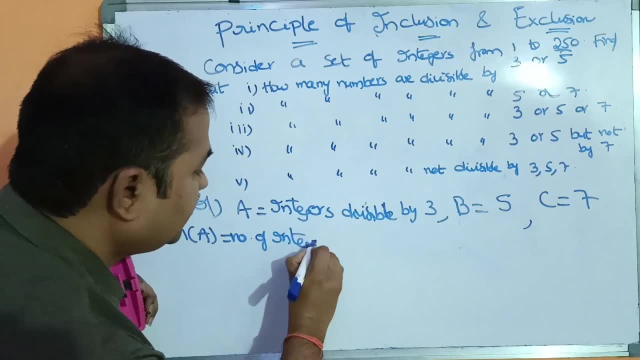 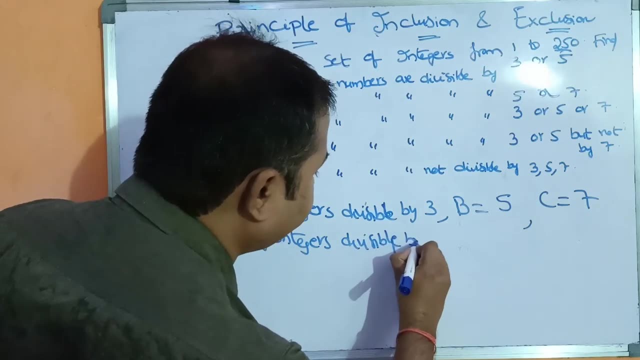 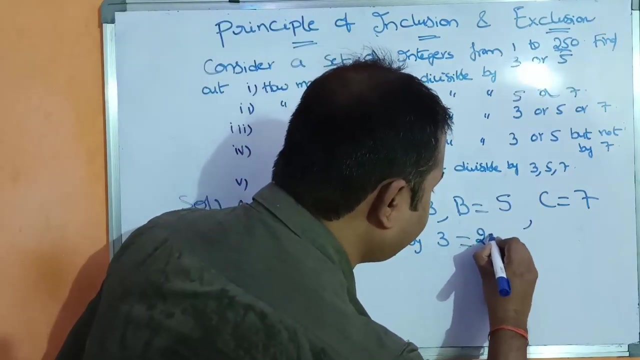 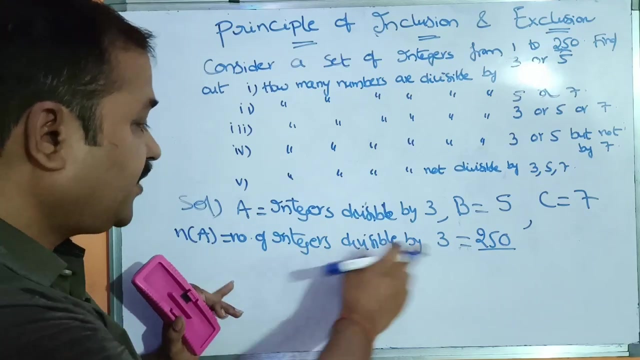 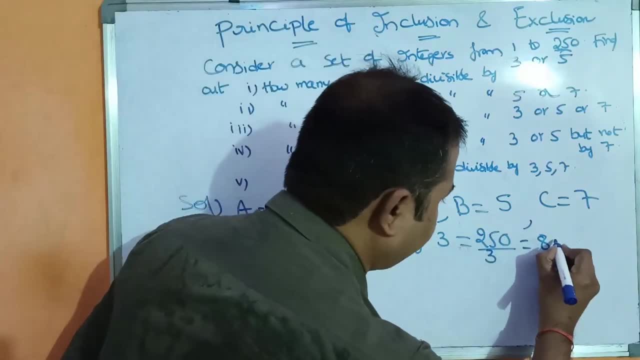 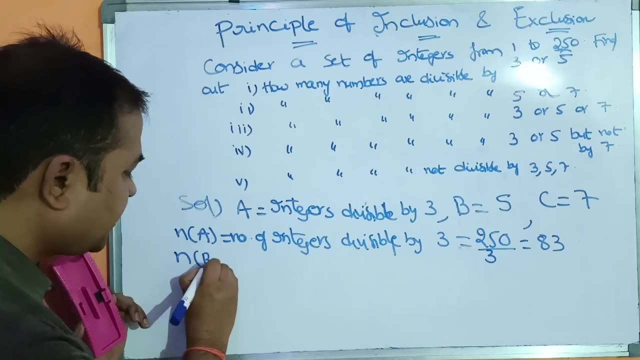 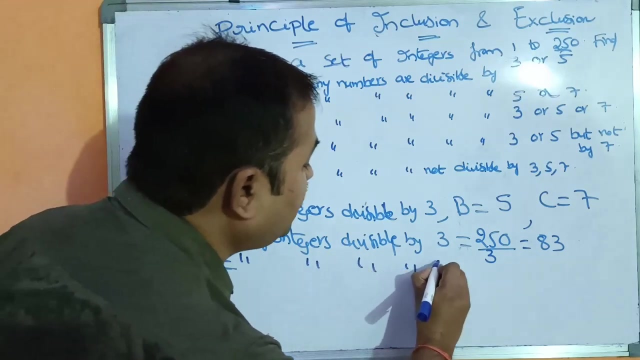 3: 8's are 24.. 3: 3's are 9.. Okay, We have to ignore the fractional part. Likewise, let us find out n of b. n of b is equal to number of integers divisible by number of integers divisible by 5.. So that is. 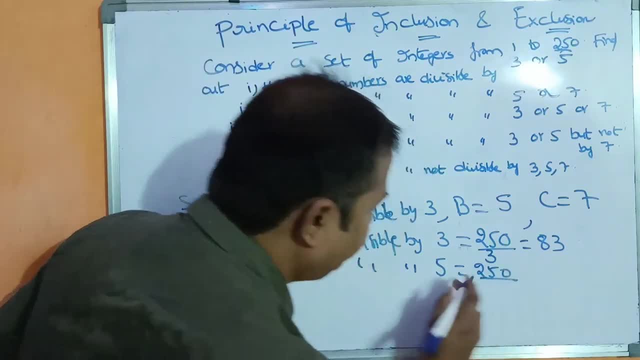 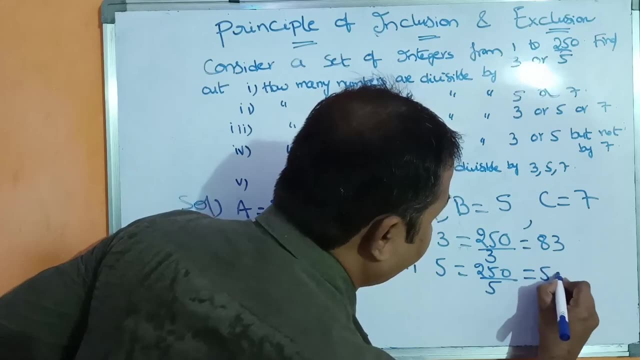 n of b. Okay, So 250 by 250 by here we are calculating divisible by 5.. So 250 by 5 means what 5 5's are? 25, 50. Next, likewise, let us calculate n of c. n of c is equal to number of. 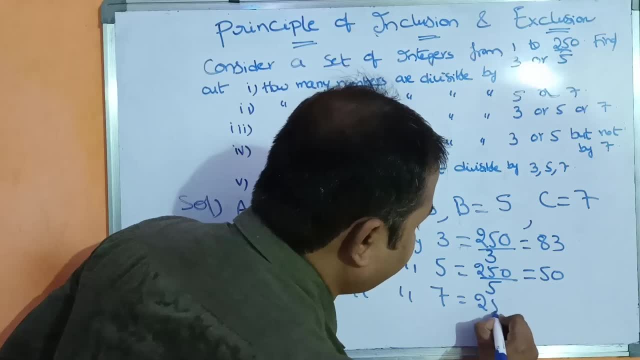 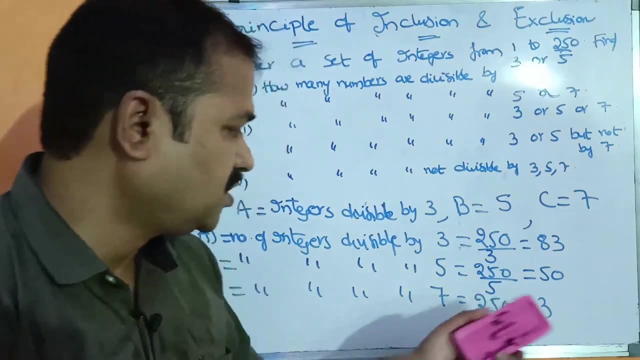 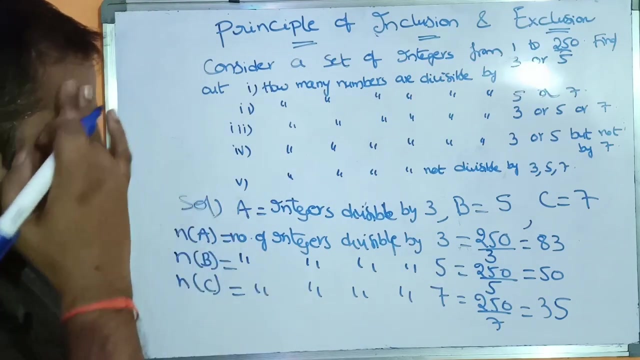 integers divisible by 7.. So 250 by 7.. 250 by 7.. So 7, 3's are 21.. Next, 25 minus 21 means 4.. So 4, 0, 35., 35. So that is what is n of a, What is n of b And what is n of c. So likewise we can calculate. 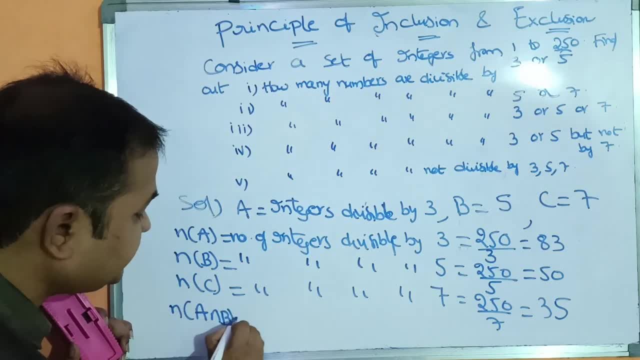 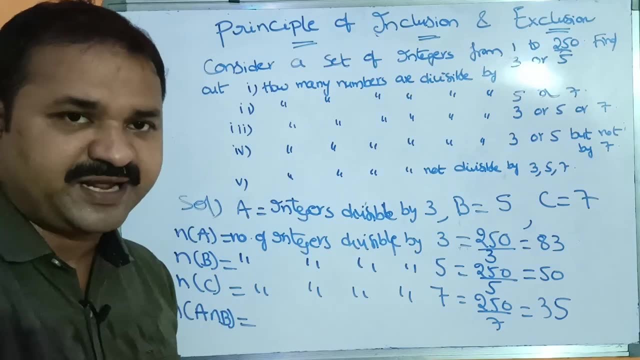 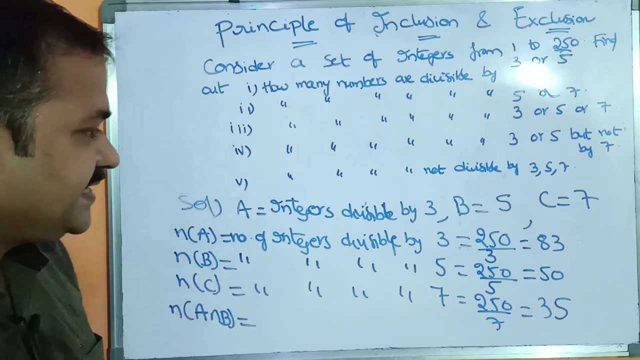 n of a intersection b. So what is n of a intersection b? Number of integers divisible by intersection means under operation. Number of integers divisible by 3, 3 and 5.. 3 and 5. That is equal to 250 by. 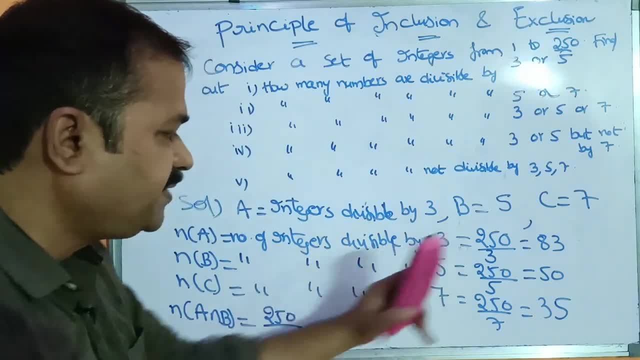 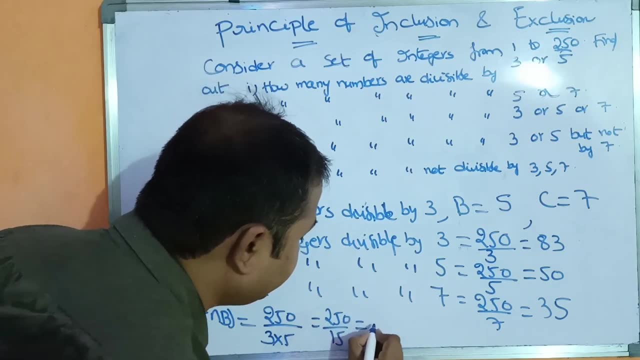 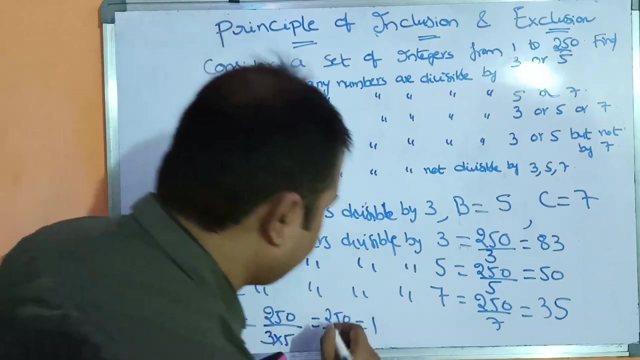 a. a means a, a means what, 3.. b means 5.. So 250 by 3 into 5.. So that is equal to 250 by 15.. So what is the result? 15? 1's are 15.. 25 minus 15 means 10.. Next 15: 100.. So 15: 6.. Likewise, let us calculate n of. 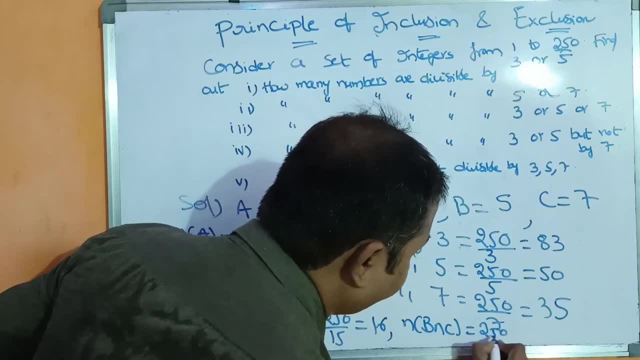 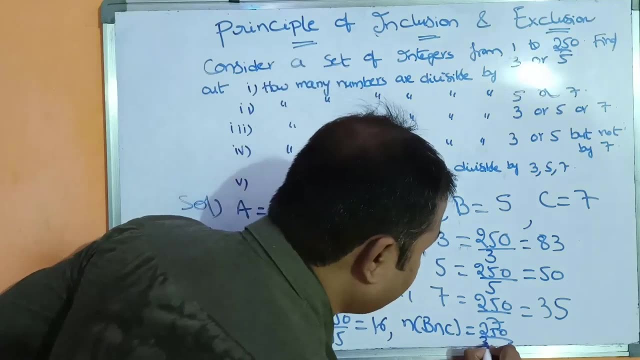 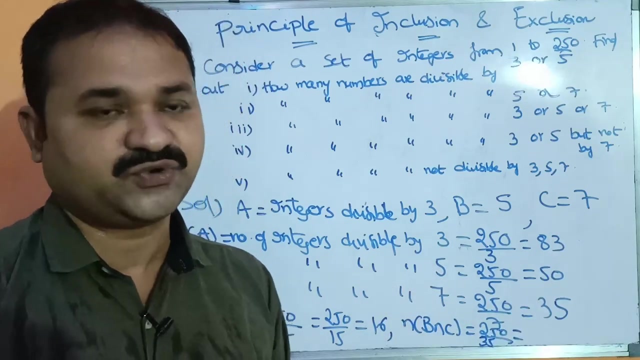 b, intersection c. also: 250 by b into c, b into c. What is b? b means 5.. Where ya, c means 5.. 15 by b into c. So 251: 0 is 252 plus 5.. Here is b. you take this multiplied by 15 is 1 and. 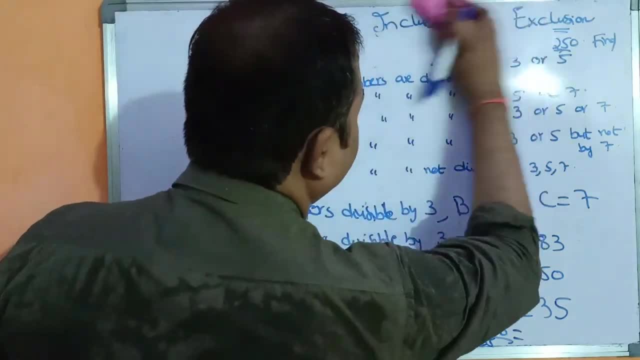 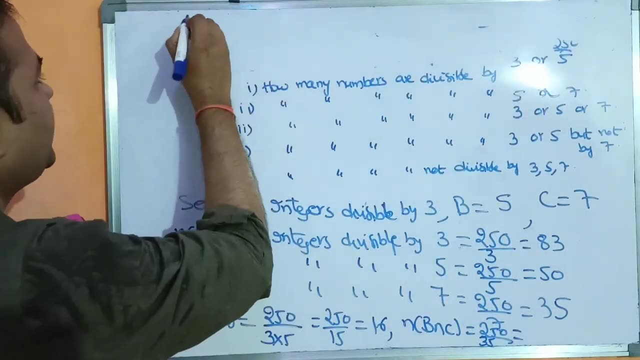 b, grade b, b into c, and see what you get. N of 0 is 0.. It is just a��만 1: 0 into 6 and you minus 4.. In this way, we are making a幅 to be 0 for the new fraction. Now N of n is equal to. 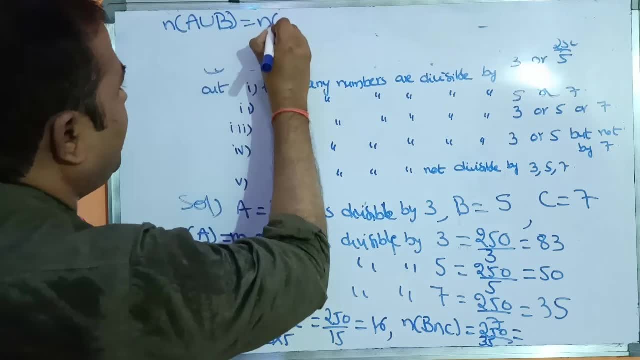 3, 수 n, 3, 3 oraz 4. 3 cancelled elsene is always 0. Therefore, n ofa union b is equal to n ofa union b is equal to n ofa union b, which means what number of integers divisible by a or divisible by b. 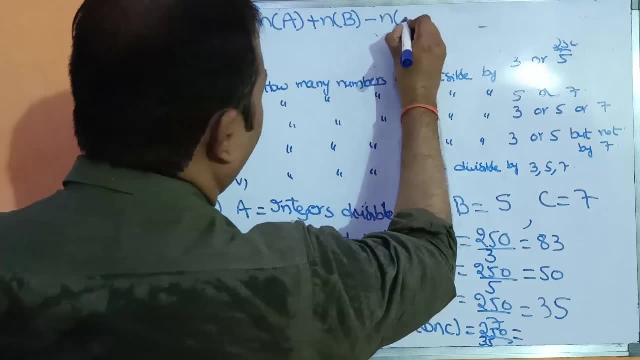 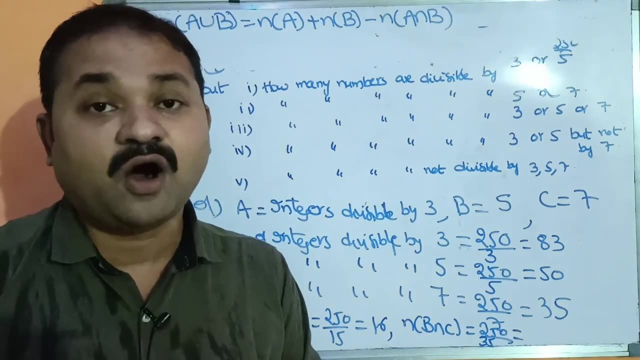 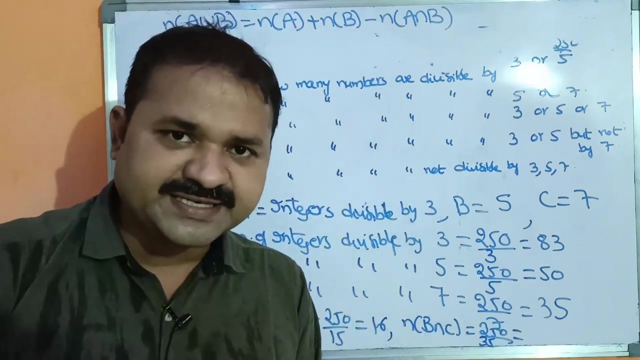 a plus, n of b minus, n of a intersection b. So what is n of a union b? Number of integers divisible by a or b is equal to n of a, means number of integers divisible by 5, n of b means number of integers divisible by b. n of a intersection b means number of integers. 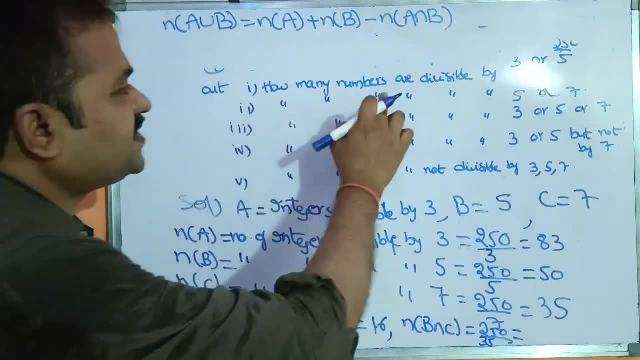 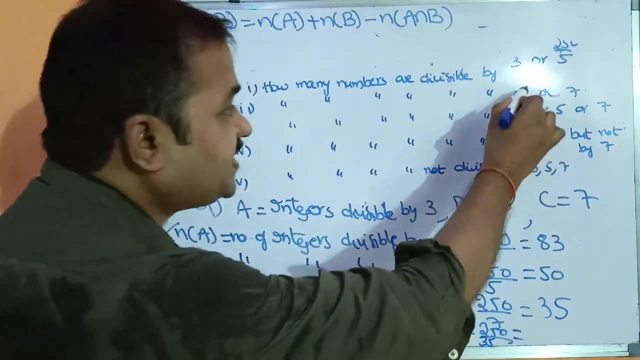 divisible by a and b. ok, Here, what is the first problem? How many numbers are divisible by 3 or 5?? Here, 3 means what. n of a Where he has 5, means what? What is the first problem? 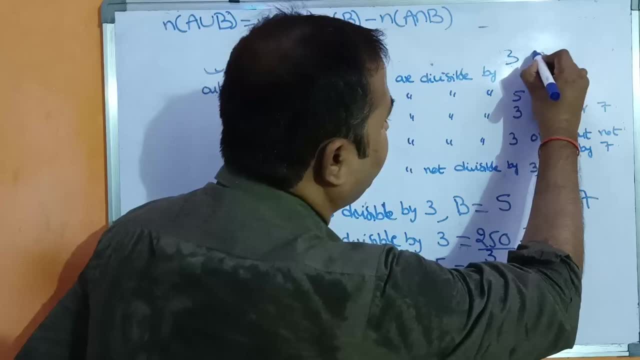 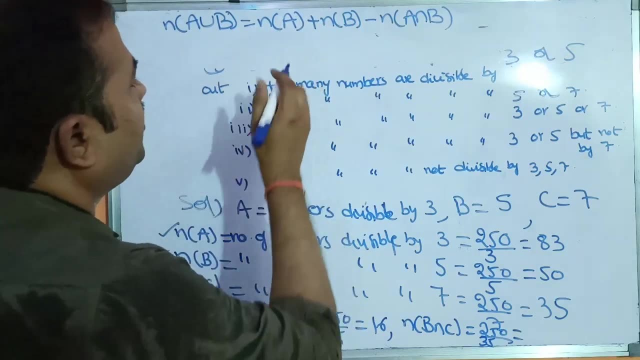 Number of integers divisible by 3 or 5, 3 or 5.. Here 3 means a, where he has 5 means b. So this is the formula: n of a union b is equal to n of a. What is n of a? 83 plus? 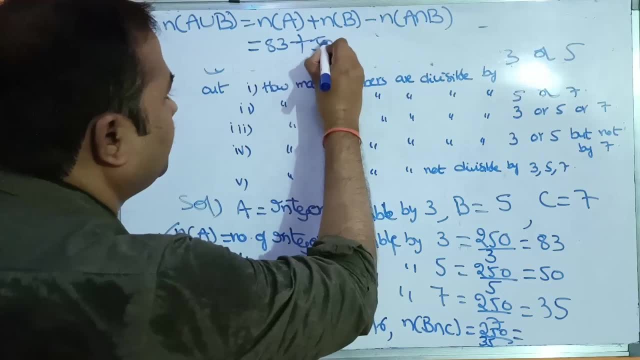 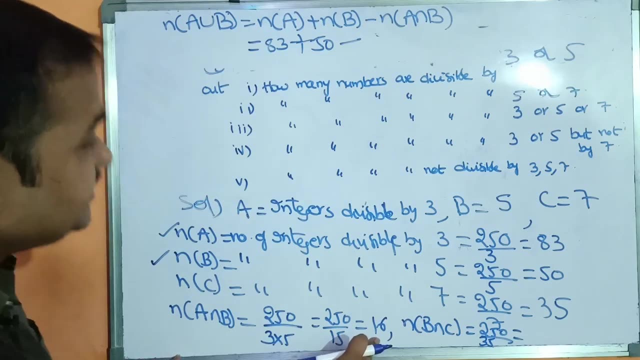 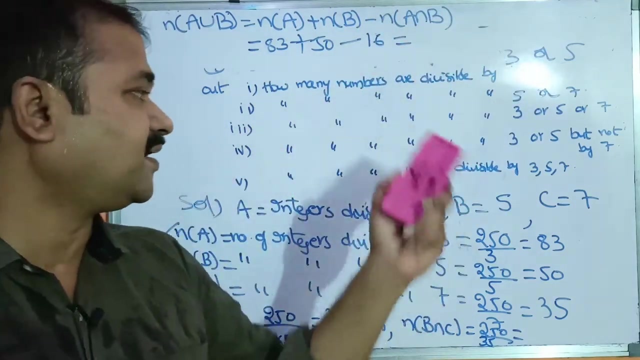 what is n of b, 50 minus. what is n of a, N of a intersection, b- Number of integers divisible by both a and b. We got the result as 16.. So 83 plus 50 minus 16.. So that is equal to some value. So that is the result. 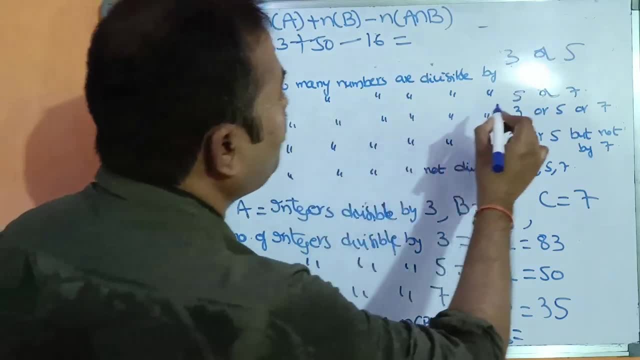 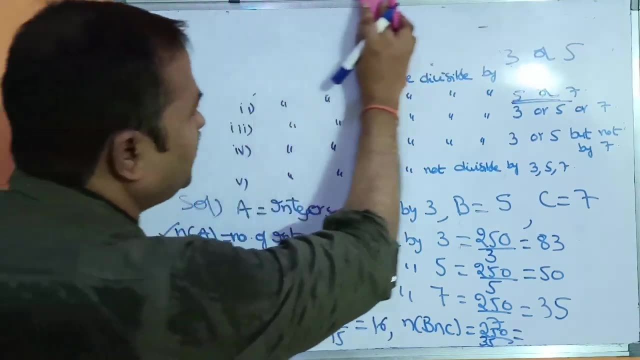 of the first problem, Let us solve the second problem. How many numbers are divisible by 5 or 7?? How many numbers are divisible by? So first problem is over. Let us solve the second problem: How many numbers are divisible by 5 or 7?? 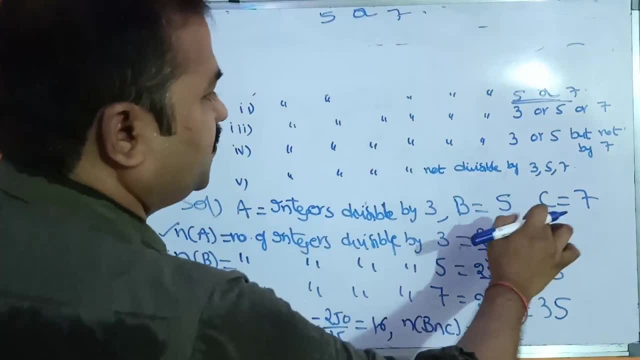 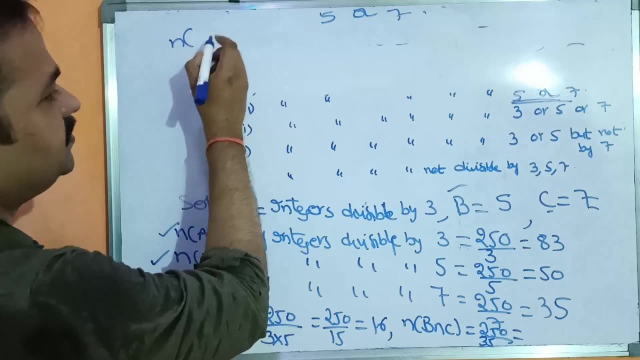 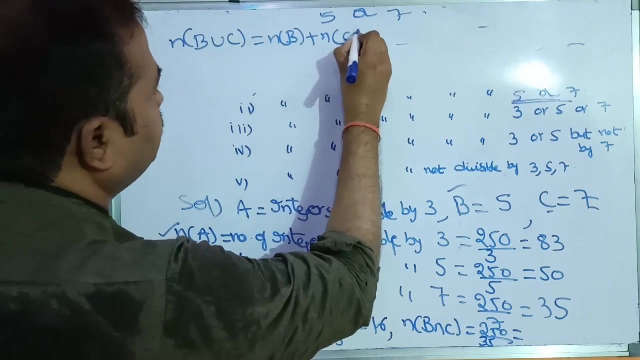 So 5 or 7.. So here, what is 5?? 5 means b value. What is 7c value? So we have to find out n of b or c. What is the formula? n of b plus n of c, minus n of b, intersection c. 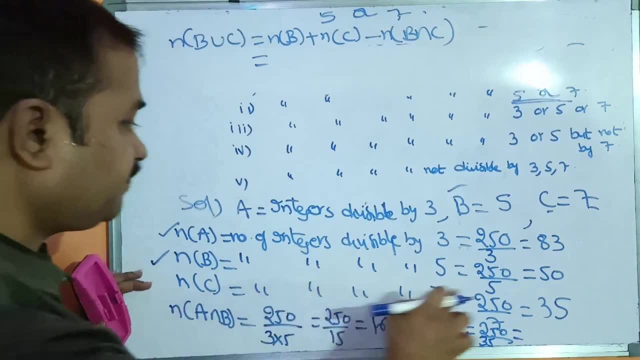 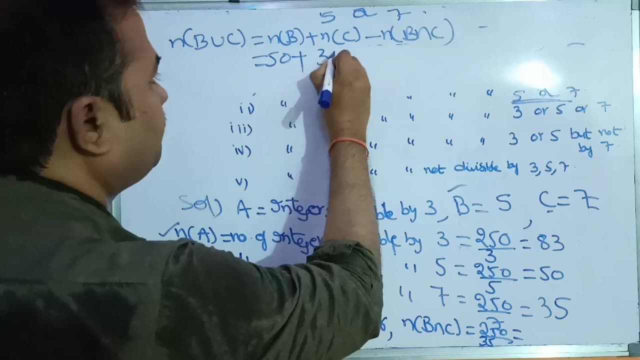 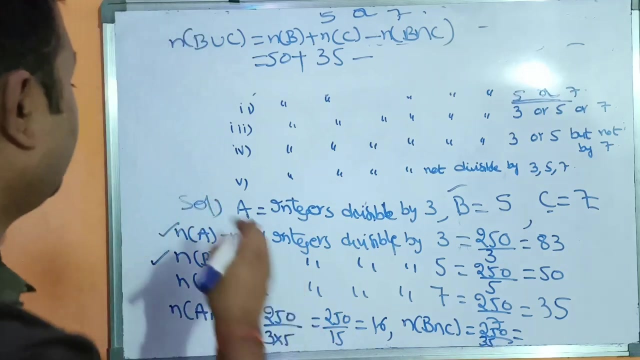 This is the formula. So what is n of b? n of b means 50 plus what is n of c? n of c means 35 minus. what is n of b? intersection c: 350 by 250 by 35.. What is the result of 250 by? 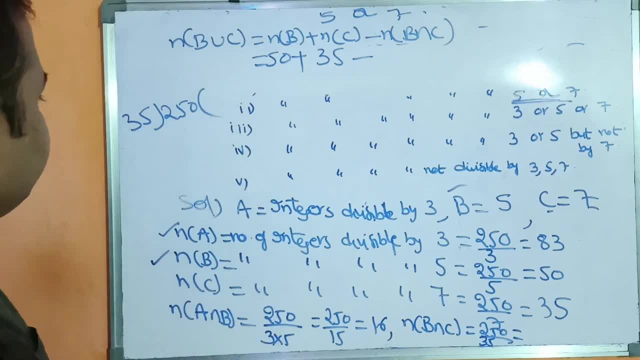 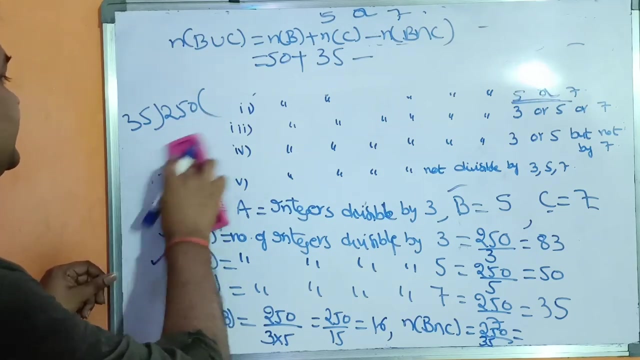 35?. So 35, 250.. So what is the result? 35, 6, 6, 6, 5 are 30.. 6, 3 is 18.. 18 plus 3, 210. So 210 plus 35 means what? 245.. So the result is 7.. So 35 into 7.. So 35. 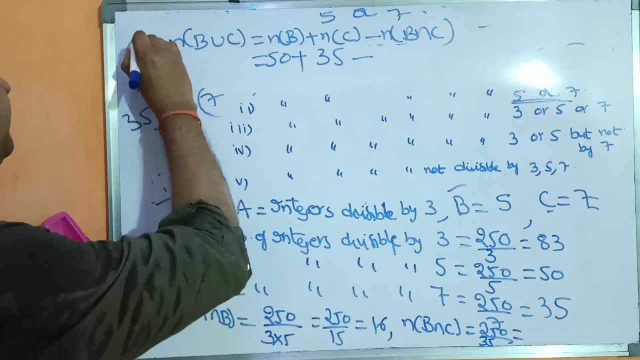 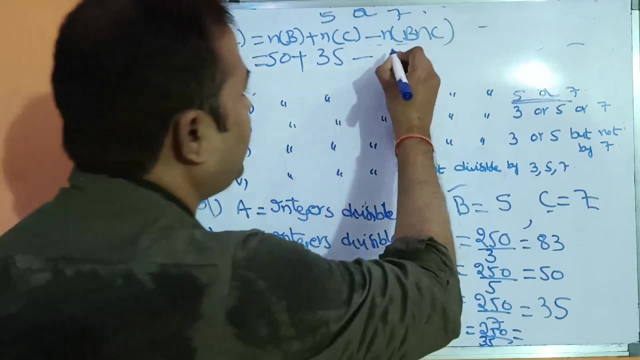 into 7.. What is the result of 35 into 7?? 7, 5's are 35.. 7, 3 is 21 plus 3, 24.. We have to ignore the fractional part. So what is the result? 7 is the result Minus 7.. So 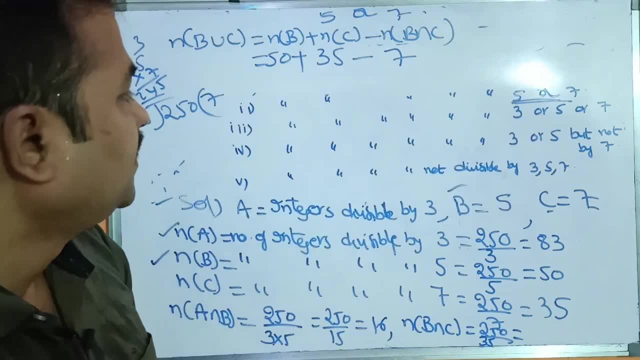 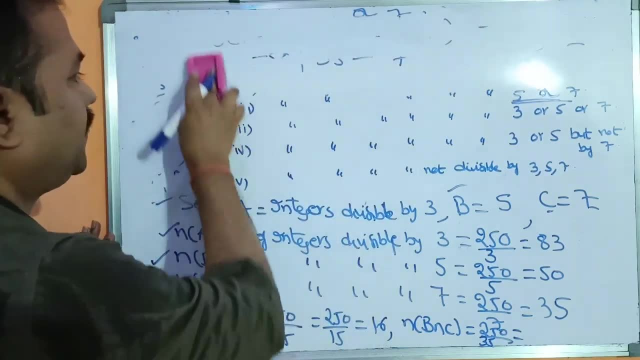 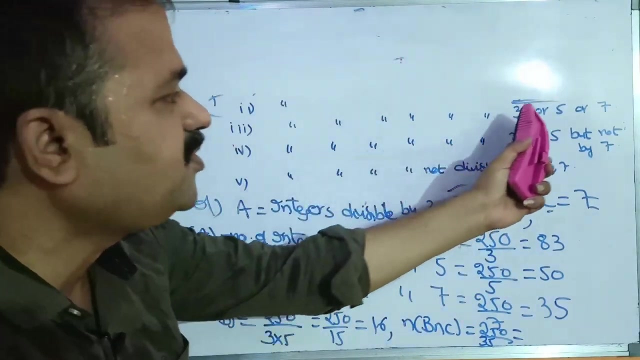 we will get some result. So that is nothing but number of integers divisible by 5 or 7.. Now let us calculate the next one. What is the next one? So second problem is also over. What is the next one? Number of integers divisible by. 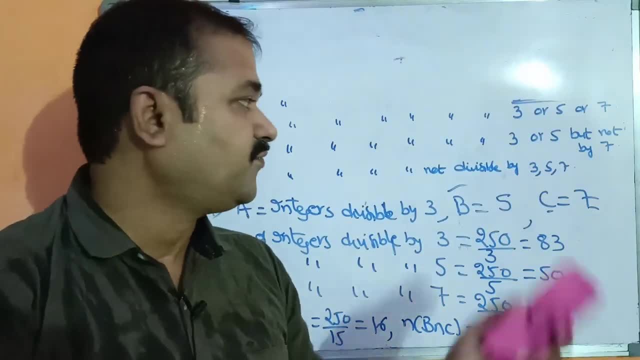 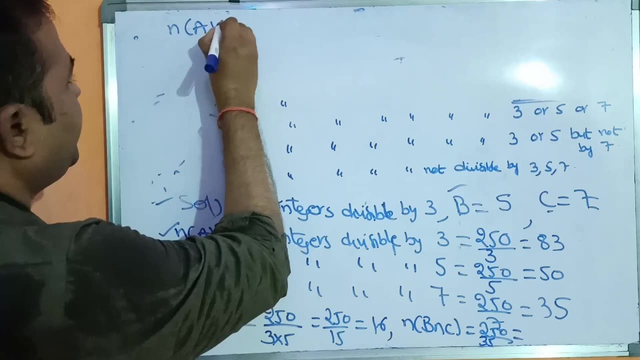 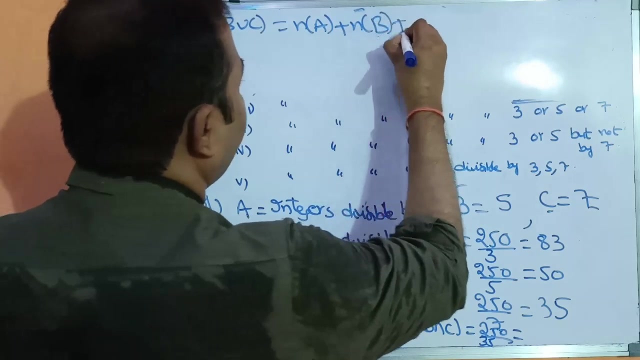 3 or 5 or 7.. So 3 means a value, 5 means b, value 7 means c, value r means union. So here the formula is like this: n of a union b, union c is equal to n of a plus n of b plus n of c. 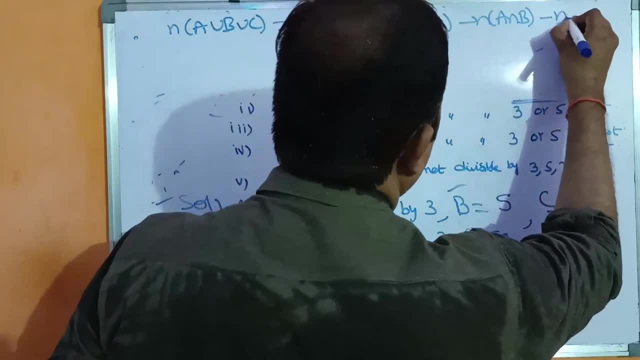 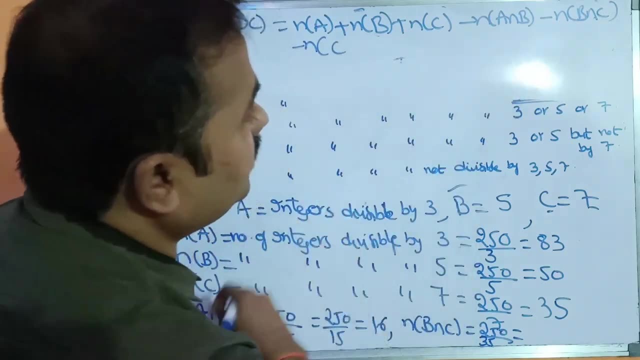 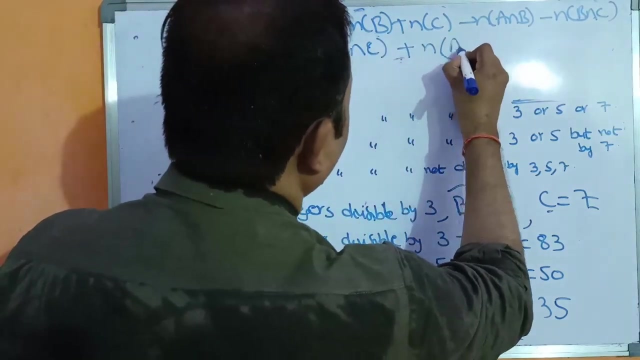 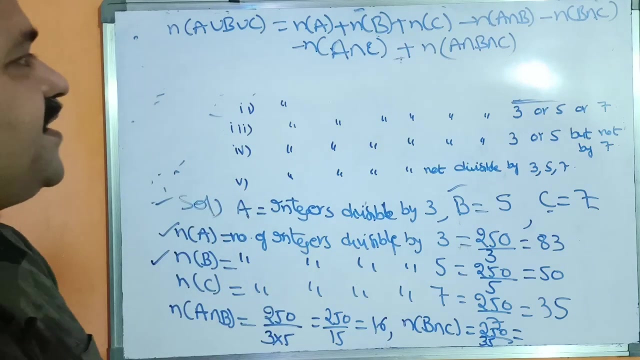 minus n of a intersection b. minus n of b- intersection c. minus n of a. b is over, bc is over. Minus n of a intersection c. plus n of a intersection b- intersection c. So this is the formula: So n of a plus n of b, plus n of c, minus n of a intersection b. 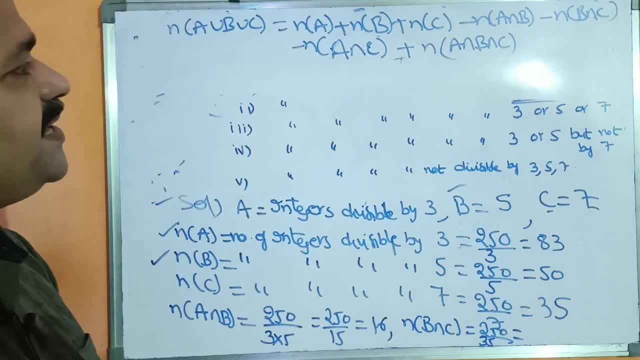 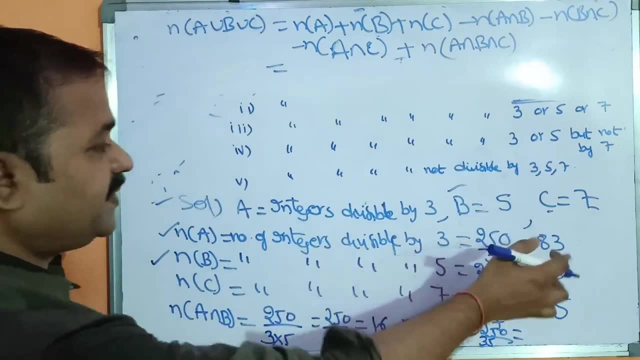 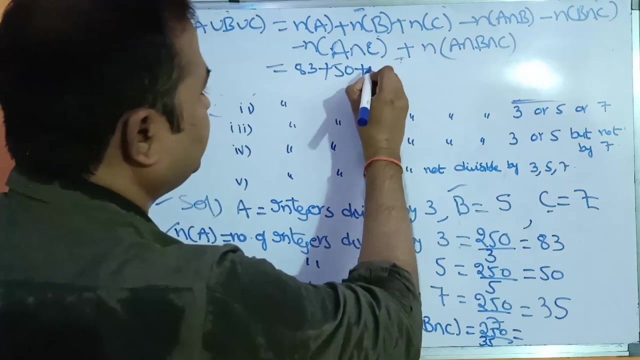 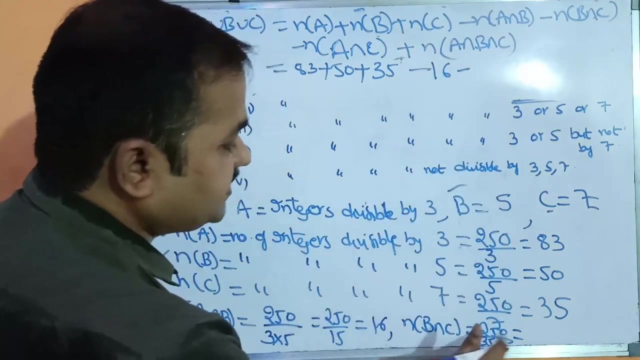 minus n of b- intersection c, minus n of a- intersection c, plus n of a- intersection b- intersection c. So what is n of a n of a is nothing but 83.. what is N of B 50 plus? what is N of C 35 minus? what is N of A intersection B, 16 minus what is? 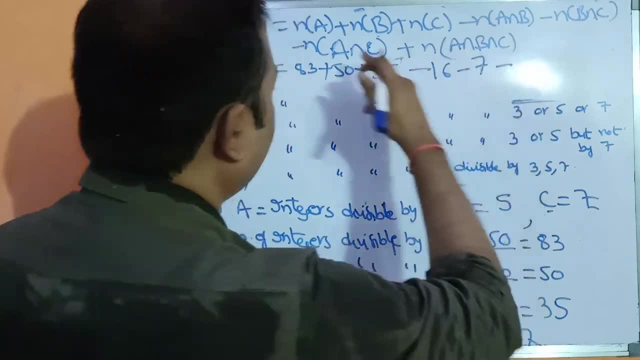 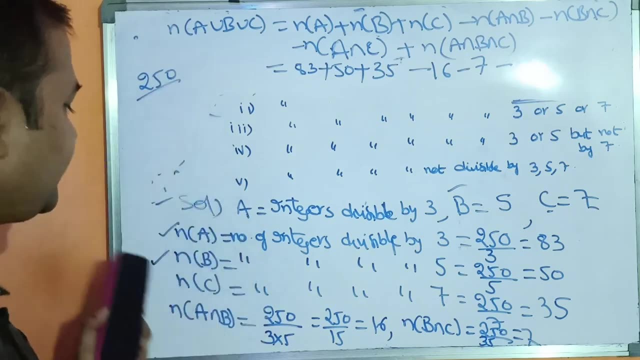 N of B intersection C- It was already calculated- 7 minus N of A intersection C. What is N of A intersection C, So 250, by what is N of A value, What is N of A value? So N of A means what? 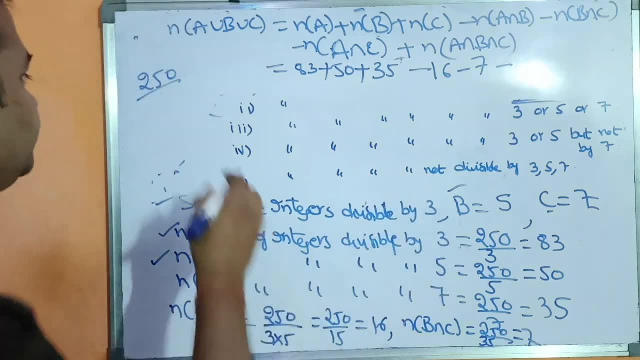 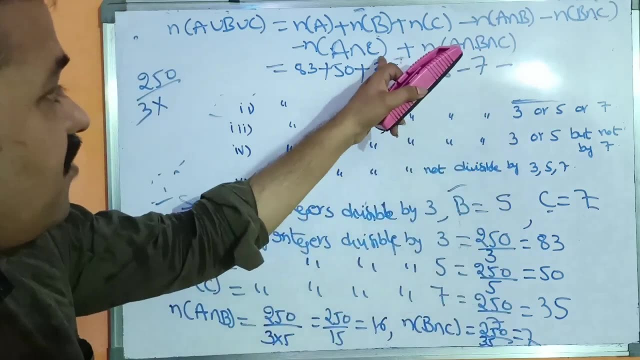 Number of integers. A value is what: 3. So 3 into this is the formula. So 3 into 250 by 3 into here we are calculating N of A intersection C, What is C value, 7. So 3 into 7 means what. 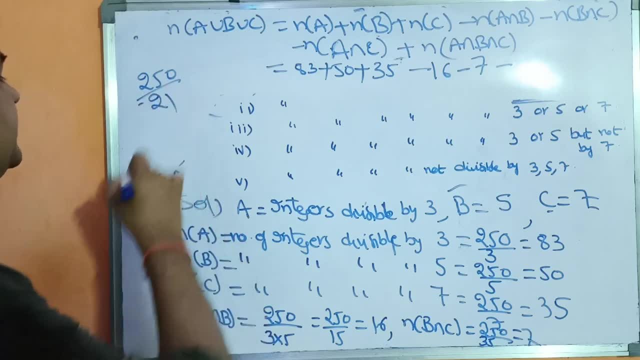 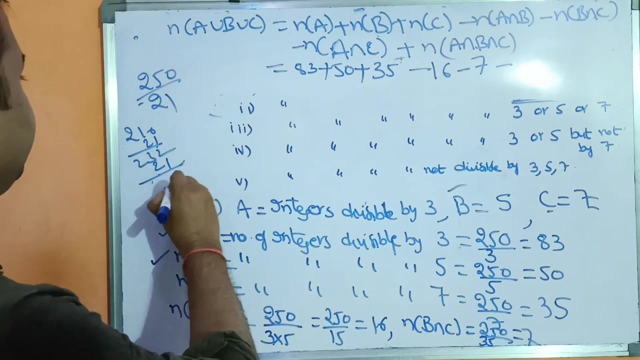 21.. So 21.. So what is the result? So 21 10s are 210.. Next, 210 plus 21 means what? 210 plus 21 means 232.. 232 plus 21 means what? So 21 is 3.. Yeah, 3 plus yeah, it is not possible. So the result is: 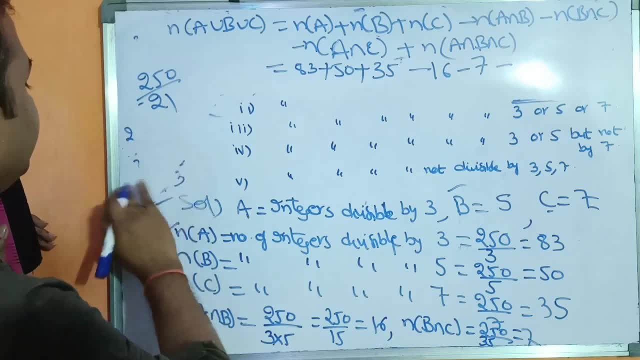 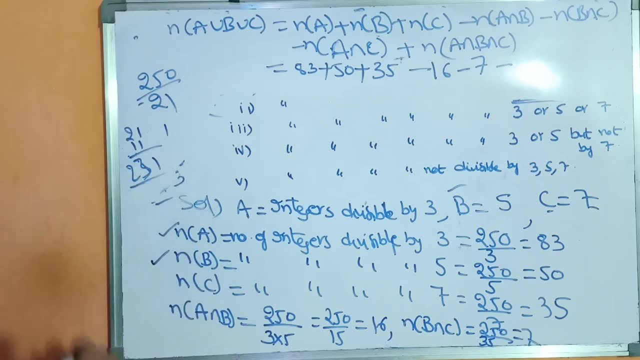 11.. So 21 into 11 means 21 into 11 means 11, ones are 11.. 11, 22 is 22.. 231.. 231.. Okay, So 11 is the result. So minus 11 plus N of A, intersection B, intersection C, So 250 by what? 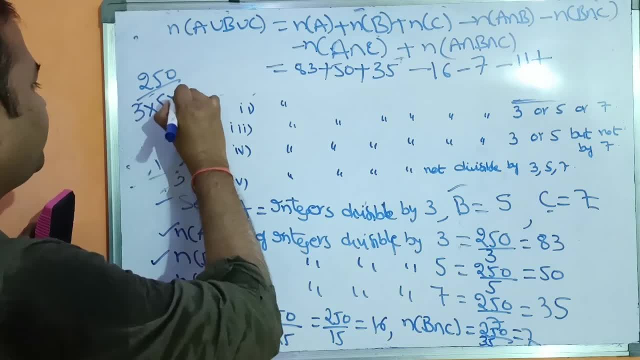 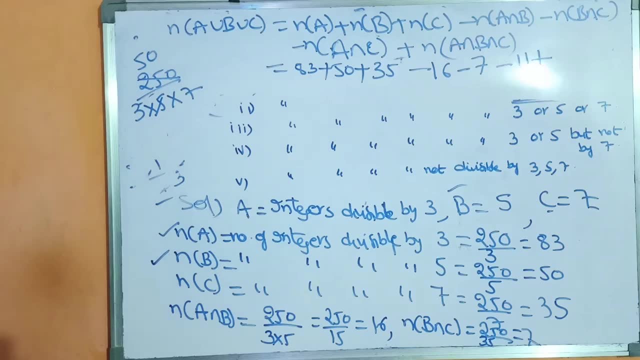 is A value, 3. What is B value, 5. What is C value, 7. So 5 into 50.. So 50 by 3 into 7.. So 50 by 3 into 7 means. 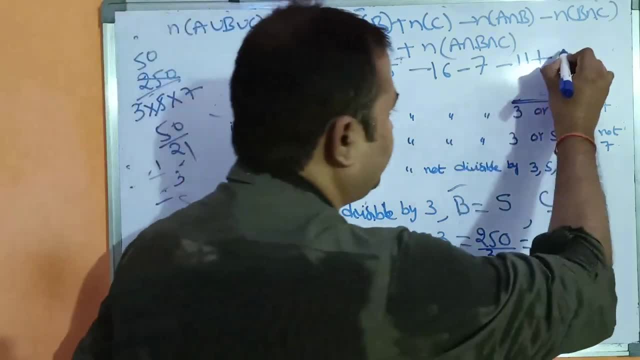 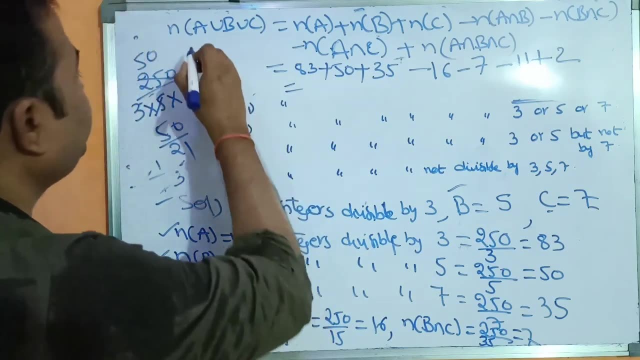 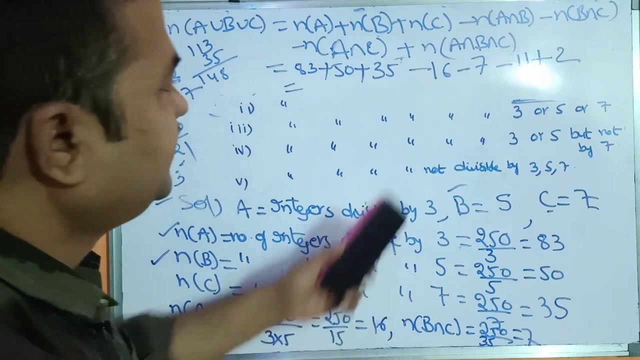 21.. 21,. 2s are 42. So 2.. Okay. So what is the result? 83 plus 50 means 113.. 113 plus 35 means 113 plus 35 means 148.. Next, 16. 17.. 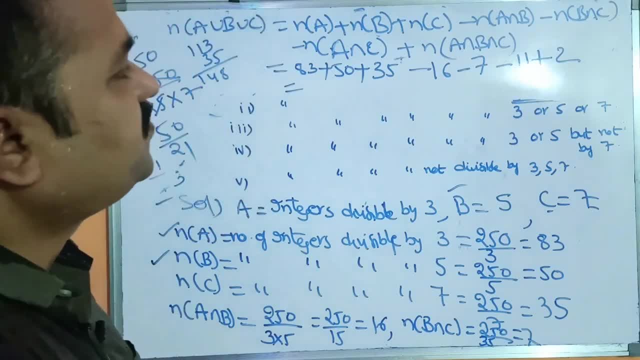 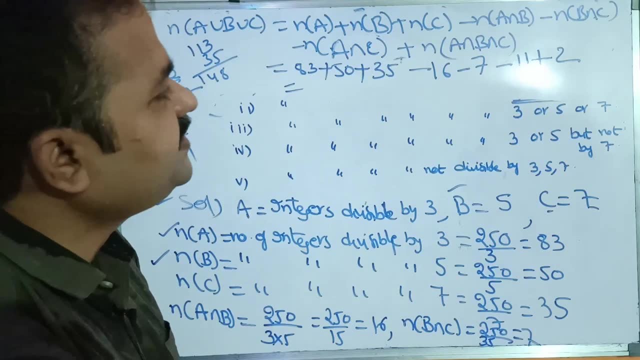 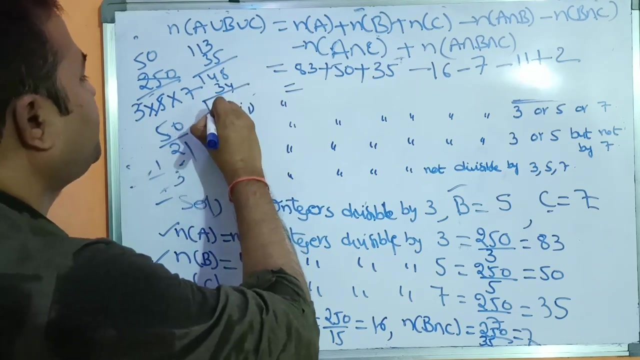 23. 23. 11 means 23.. So 16 minus of 16 plus 7, 23.. 23 plus 11 means 34.. So 34.. So 148 minus 34. So that is equal to 114.. 114.. 114 plus 2 means what? 116.. So this is the. 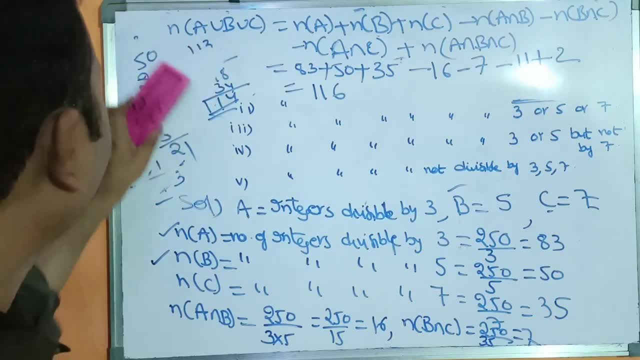 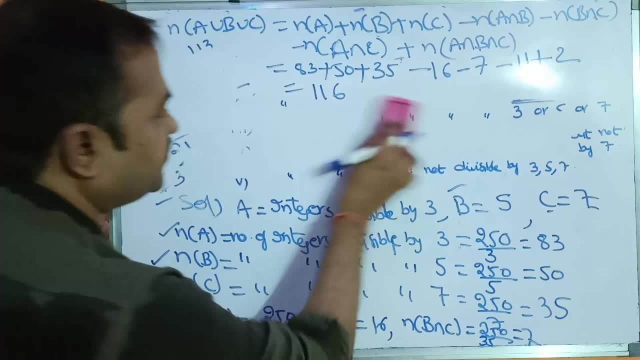 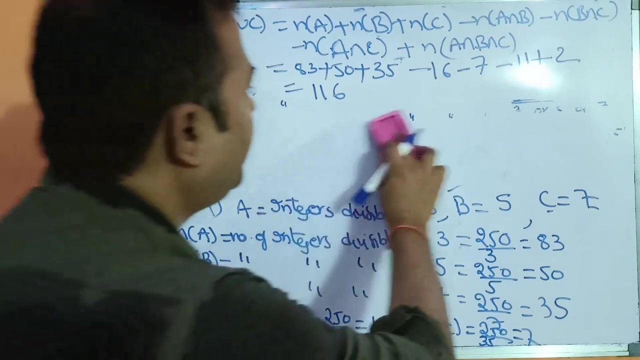 result. So what is the result of N of A union B, union C: 116.. 116 is the result. Okay, Likewise, let us solve the remaining problems. So what is the next problem? What is the next problem? Number of integers. Number of integers divisible. 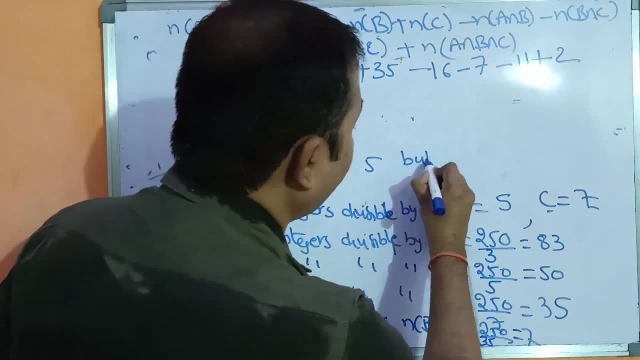 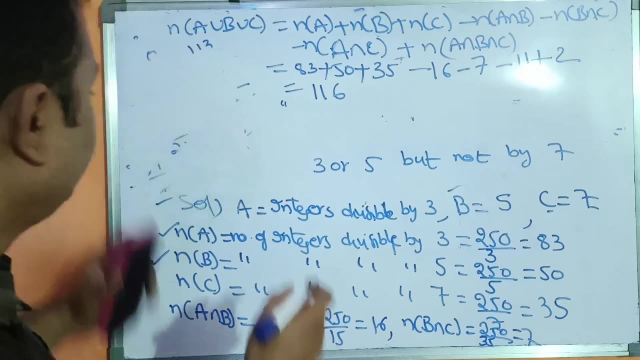 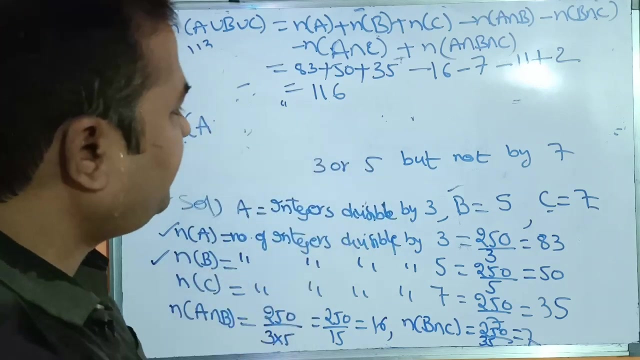 by 3 or 5,, but not by 7.. Number of integers divisible by 3 or 5,, but not by 7.. So let us see this problem. N of 3 means A value R N of here we need to find number of integers divisible by 3 or 5, but not by. 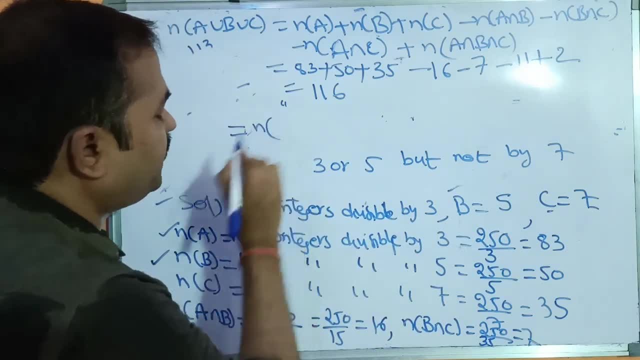 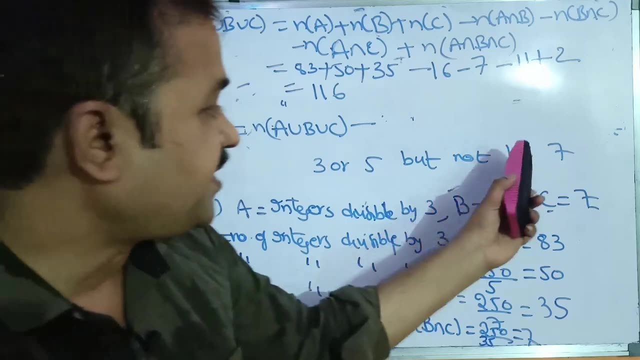 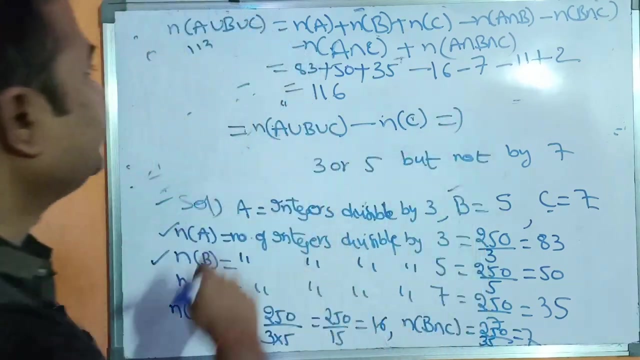 7.. Okay, The formula is very, very simple: N of N of A union B union, C minus, but not by 7, but not by 7.. 7 means C value, So we have to subtract with C. So what is N of?